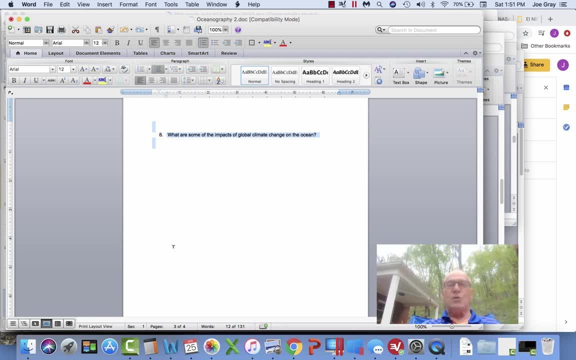 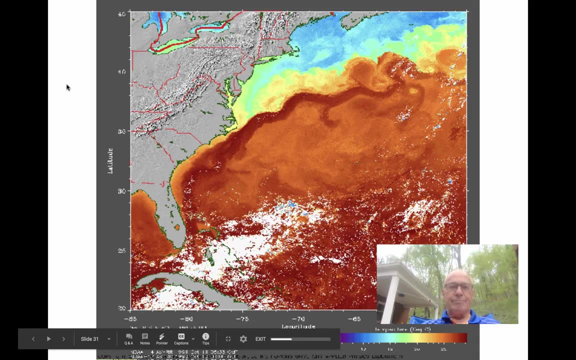 information. This will complete what you need to turn in by next Wednesday. So let's take a look at what exactly currents are. Here we see a temperature view photograph, basically like a satellite view of the ocean surface, And the red colors indicate warm water and the blue colors indicate 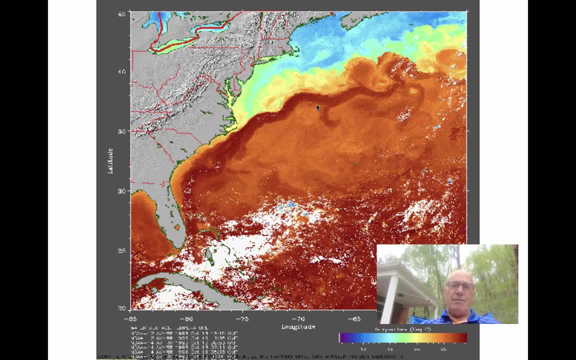 colder water. Well, right here you can see this pattern, right here this nice warm water, And this is an example of a current right. This is a specific current known as the Gulf Stream, which sweeps past the eastern part of the United States and actually moderates and keeps our 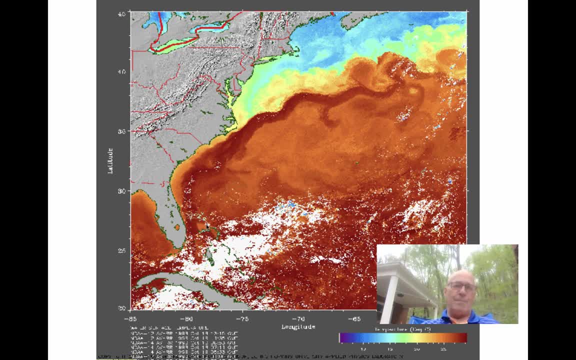 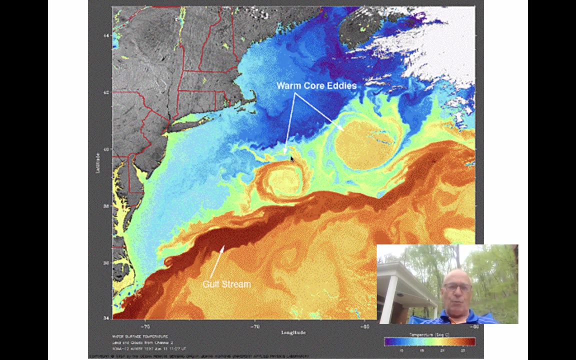 temperature fairly mild. If we had a current going in the opposite direction, we would have much colder winters, much milder summers, probably much less springtime. We'd have much cooler weather. Right here you can see these currents right here called warm core eddies. So you can see where these water, this water, is broken. 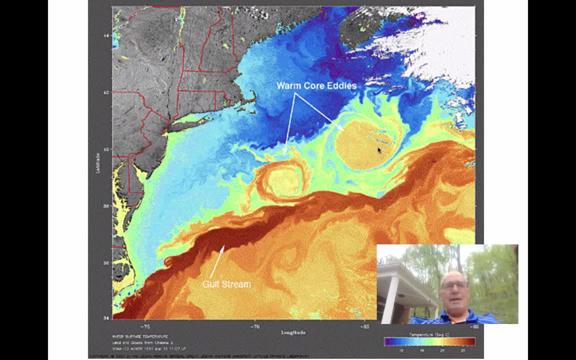 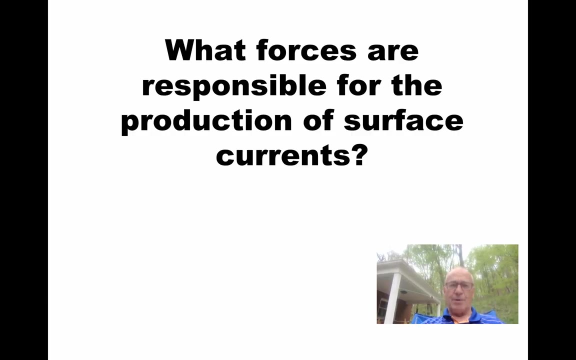 off of this mainstream, creating these little swirls. You might have seen something like this in a creek or stream, or if you've gone down to Lake Cumberland, you'll see these, where water mixes in creating these currents. So exactly what causes ocean currents? right, What? 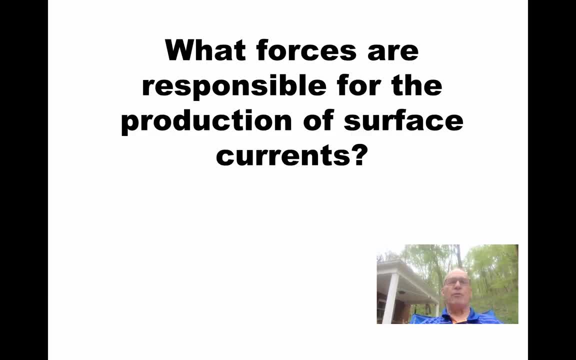 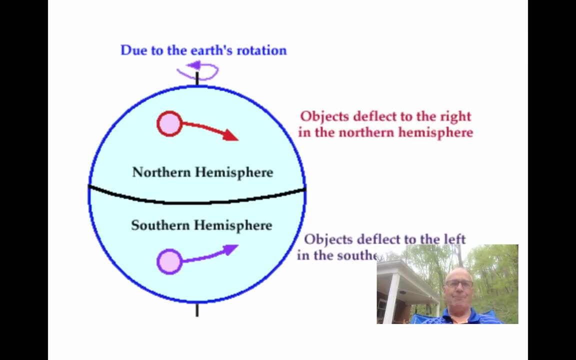 forces are responsible for the production of ocean currents? This is your first question. And the two forces that are at work that are responsible are wind and what is known as the Coriolis effect. Now, what the heck is the Coriolis effect? Let's talk about that. 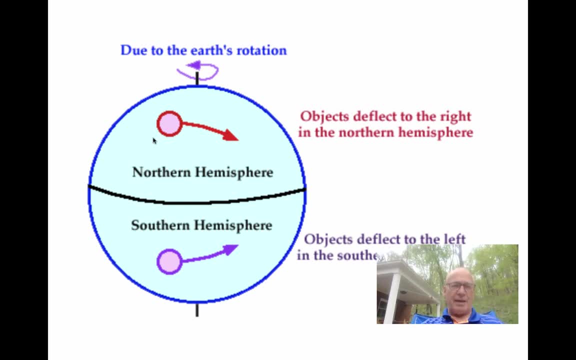 The Coriolis effect causes this to happen. So you have wind being produced here in the Northern Hemisphere, But that wind is affected by the Earth's rotation. Now our rotation is counterclockwise right here If you're looking down on the North Pole. 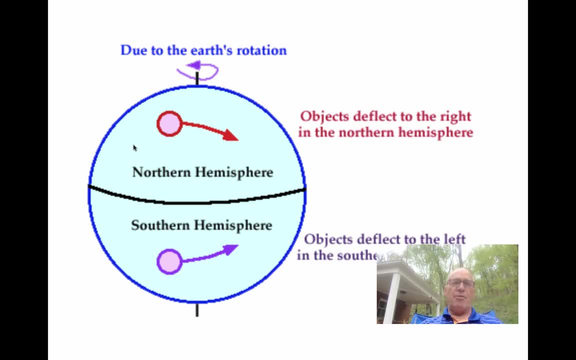 so you have counterclockwise rotation And what that does is that deflects all the wind and therefore all the water to the right in the Northern Hemisphere. Objects are deflected to the right in the Northern Hemisphere And then that would be to the left in the Southern Hemisphere. 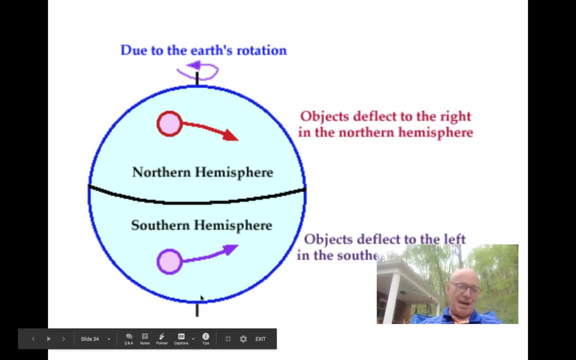 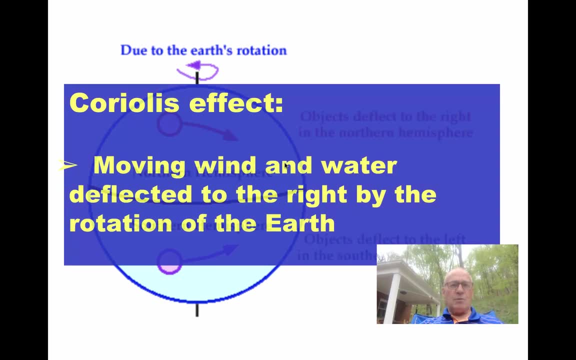 based on that, That's your right. But if you're standing on the South Pole looking in the opposite direction, picture yourself upside down here. that would be to the left. So here's your vocab term for Coriolis effect: Moving wind. 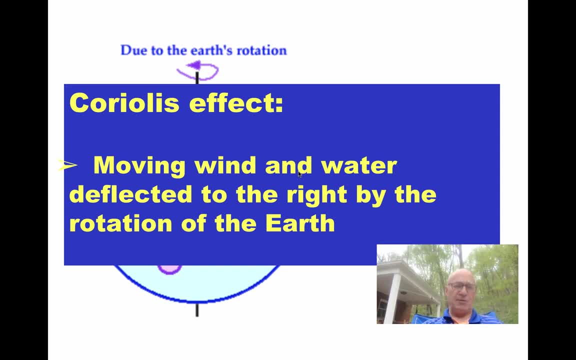 and water are deflected to the right, that's, in the Northern Hemisphere, by the rotation of the Earth. Let's take a look at a video clip that, hopefully, is going to help us understand that a little better. So here you see, these two people stationed on this merry-go-round throwing a ball. 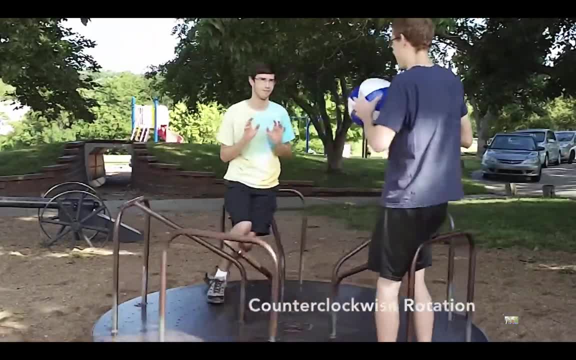 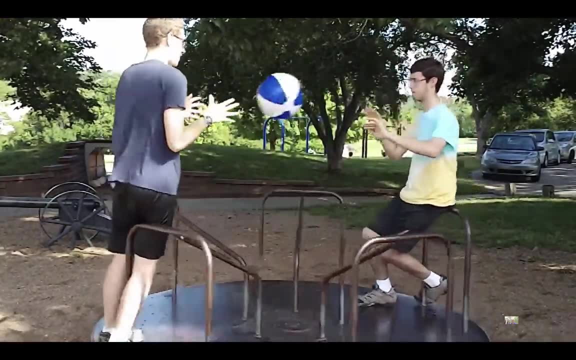 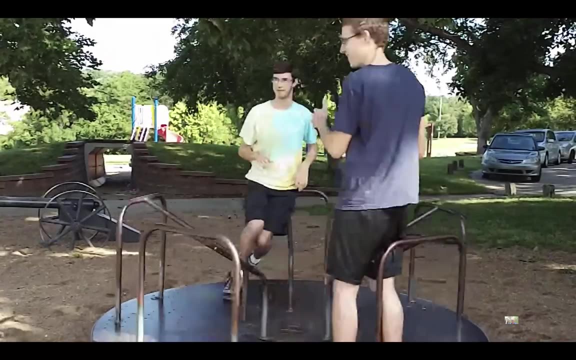 You can see. it's pretty clear. They can throw the ball straight back and forth. Now watch what happens when they're rotating counterclockwise. That first guy is still throwing the ball directly at the guy across from him, but the ball curves to the right. This is because the second person is basically 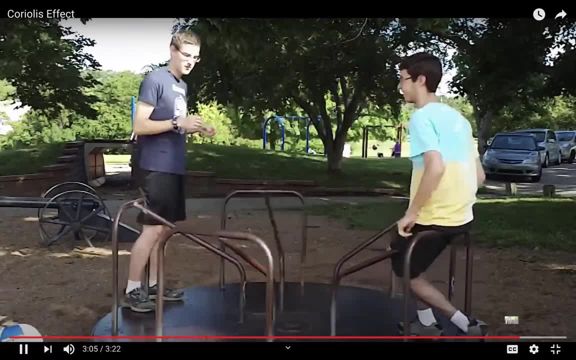 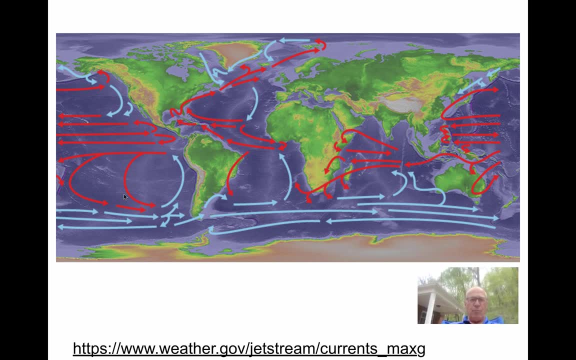 moving away from where the ball would have been going, And that's what's happening to the wind. So here is the effect, then, that this has on the world's oceans. Again, we're focused on oceanography In our Northern Hemisphere, right here. 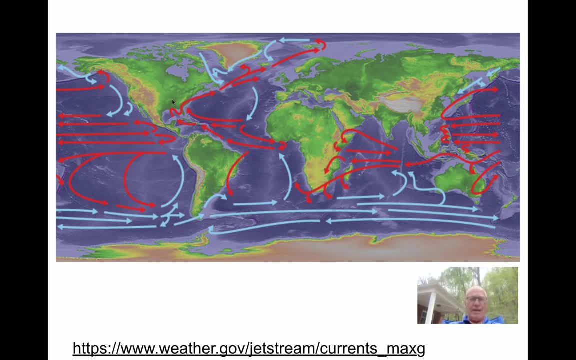 everything's getting thrown to the right, You see here, to the right in this picture. That is why our wind patterns and weather typically comes from west to east across the United States, And then that hits the water and drives it eastward as well. Now that water continues. 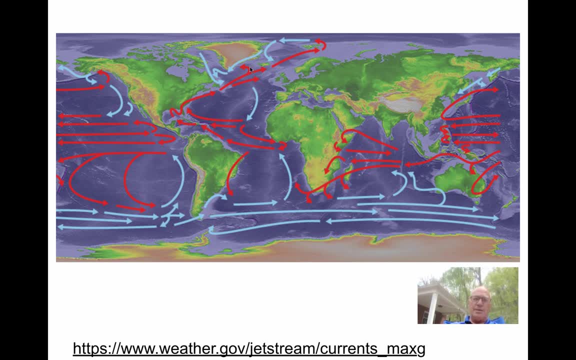 across the Atlantic- here, for example- until it hits the continents or swirls around up into the Atlantic And then it curves back. And what you're seeing in this picture right here: the red indicates warm water currents, The blue indicates cold water currents. So we have this nice warm. 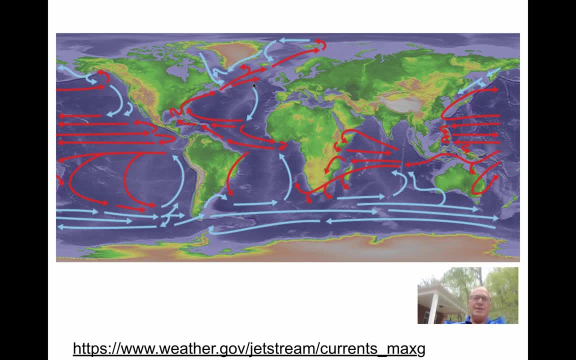 water current here, the Gulf Stream going past the United States, And then you have a cold water current curling back around to the equator where it warms back up again and swirls around. So we have a circular pattern being created here In the Southern Hemisphere. this works counterclockwise. 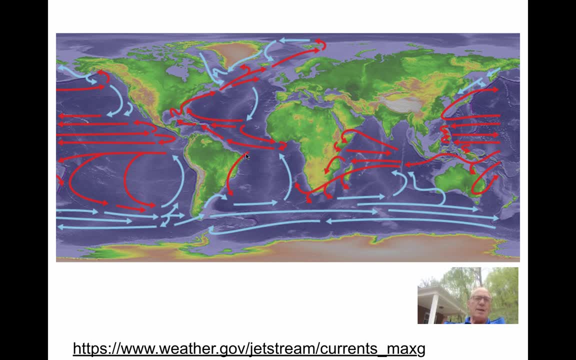 Now we've got it moving the opposite direction. right here You have this warm water current sweeping from the equator down past Brazil, in South America, And then it gets down near the Antarctic, right here towards the Southern Ocean, And that becomes a cold water current then And 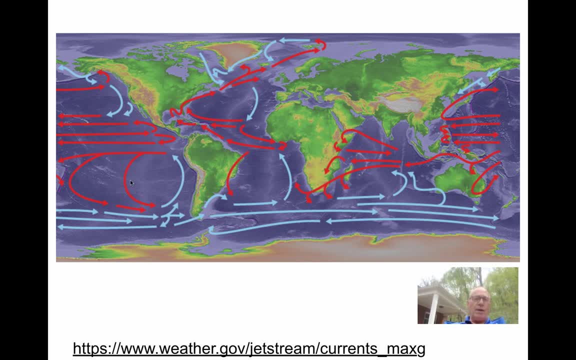 it sweeps back up this way And then you have the same thing going on over here in the Pacific. Again, it's going counterclockwise. Clockwise in the Northern Hemisphere for our currents, Counterclockwise in the Southern Hemisphere Because, again, the moving wind and water 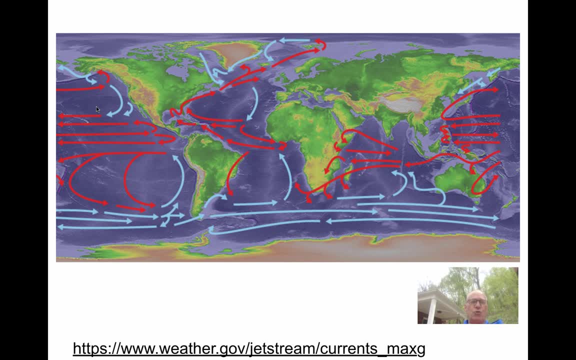 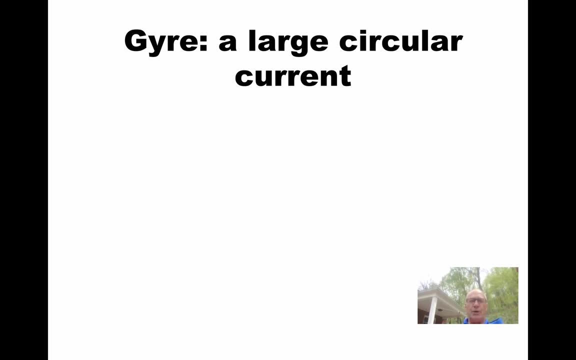 due to the Coriolis effect, is being thrown to the right. So these create what we call gyres. That's your next vocab term. A gyre is a large circular current. Now we have five major ocean gyres. This is one of the questions that you need to answer. So let's take a look at those five. 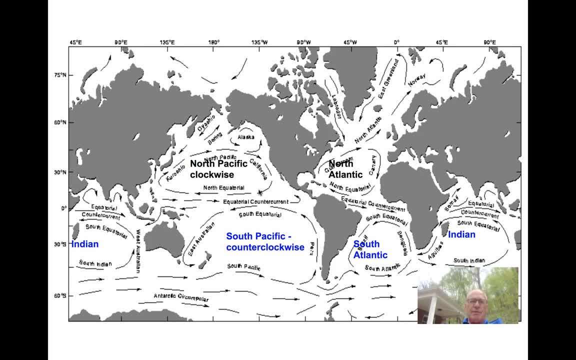 major ocean gyres. The first that we're going to talk about is the North Pacific And again, you can see, this is a clockwise current. right here In the South Pacific we have a counterclockwise current. So those are your first two: North Pacific, clockwise South Pacific. 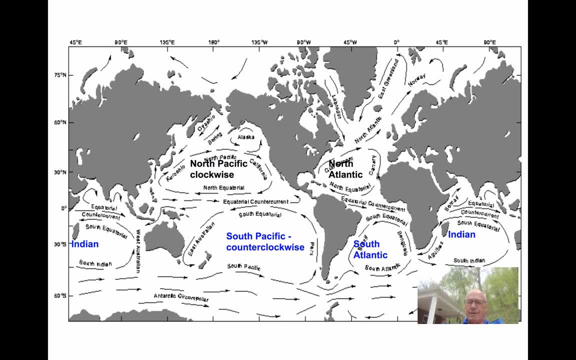 counterclockwise. North Atlantic clockwise, South Atlantic counterclockwise. And then there's the Indian gyre And that's also counterclockwise. So you have three counterclockwise gyres right here: South Pacific, South Atlantic and the Indian gyre, And then two clockwise. 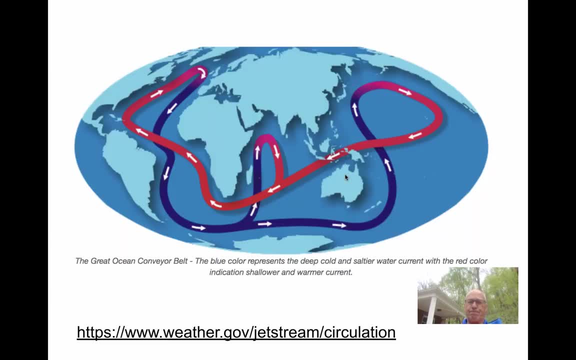 gyres, the North Pacific and the North Atlantic. This is affected by an overall circulation of water Which is known as the global conveyor belt. right Here we have a Pure Water Belt. the Jul haciendo Salut This banked" eters. 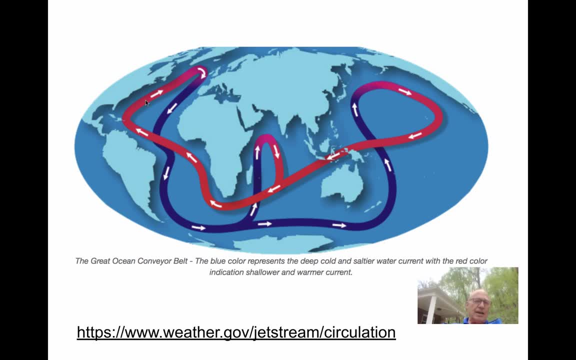 we see this warm water right here, circulates up and then comes back around this way. Now, what this is indicating is this warm water, Warm water, is lighter, just like warm air is lighter and rises. as you learn in fifth grade, This warm water stays near the surface, but as it gets up, 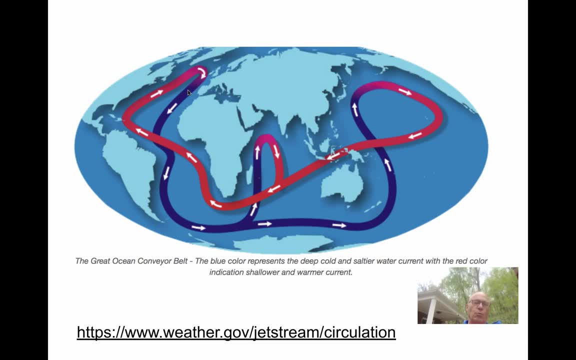 here near the poles, it starts to get cold and that causes it to sink. Cold water is heavier. Colder water- the molecules of the water are closer together, so it's heavier, So it sinks. it goes down underneath and then circulates back around the world like this and eventually rise from as it's. 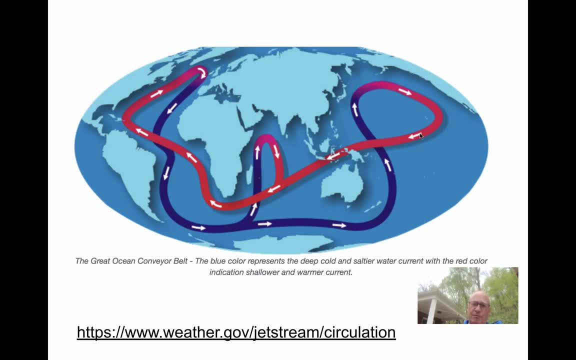 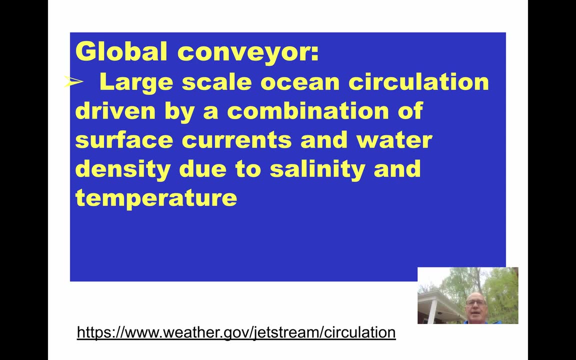 getting near the equator right here and getting warm, it rises back up to the surface, creating this thing called a global conveyor belt- That is a vocab term. This is a large-scale ocean circulation and this is driven by a combination of those surface currents that we looked at, the gyres. 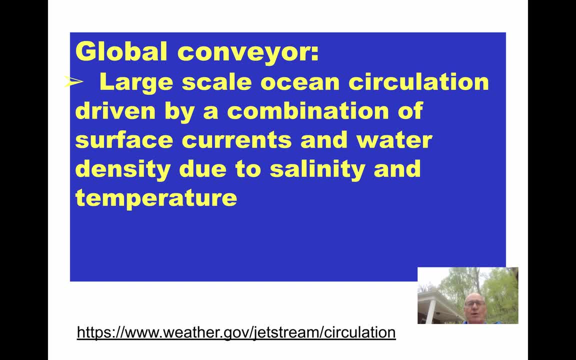 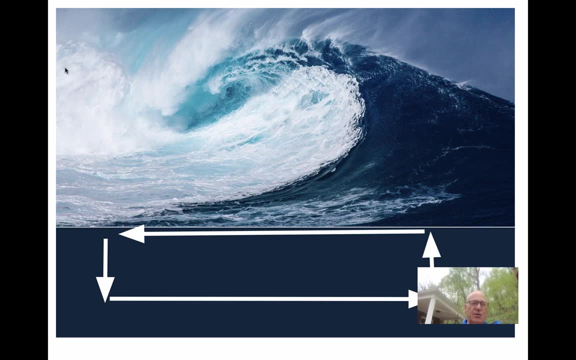 and the water density, how heavy the water is due to both the salinity and the temperature. Let's take a look at what that is all about. So here's what's happening right here: Water gets cold. Okay, let's say this is near the poles. right here, Water is also getting turned into ice. Now. 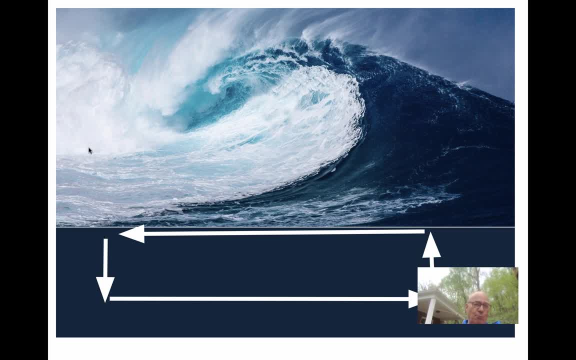 ice typically doesn't have much salt in it. When water freezes, it's just the water that freezes. the salt's left behind. Well, that leaves this remaining water right here. It has more salt in it, It's saltier, it's colder, it's saltier and therefore it's heavier and it sinks. So it goes. 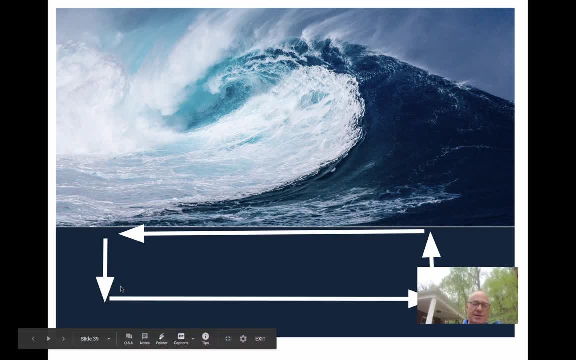 down along the bottom of the ocean here towards the abyss, travels along the abyss and then eventually, maybe, it hits a continent, so it can't travel any further and that drives it upward. Now it's near the equator, let's say, and that water is warmer. 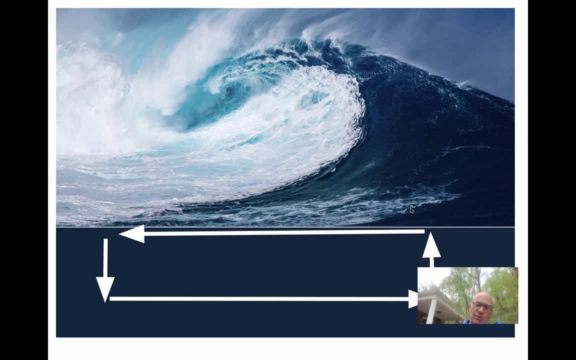 And here's your wind currents, wind-driven currents, right here pushing the water back across the surface. So we get this circulation Deeper, heavier, salter, saltier, colder water and, near the surface, a little less salty, warmer water, And that again is our global conveyor belt. 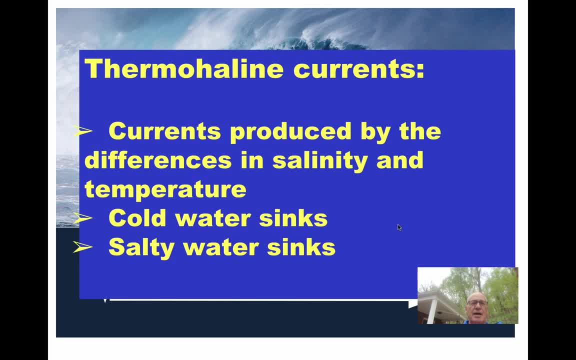 This is also known as a thermohaline current, another vocab current term. These are currents produced by the differences in salinity and temperature. Easy way to remember it again is: cold water is heavier, so it sinks. Salty water is heavier, so it sinks. Water near. 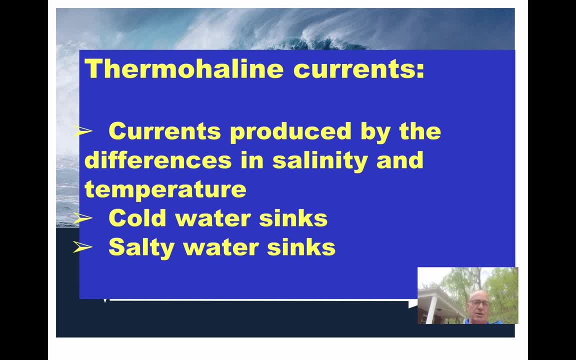 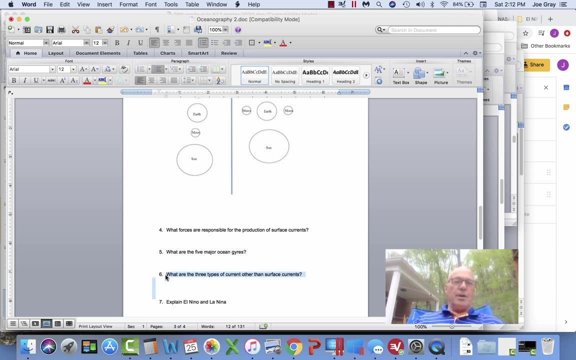 the poles tends to be colder and saltier, so it will tend to sink. Water near the equator tends to be warmer and less salty, so it tends to rise near the surface. That takes us now to question number six, right here: Three types of current other than the surface current, So the surface. 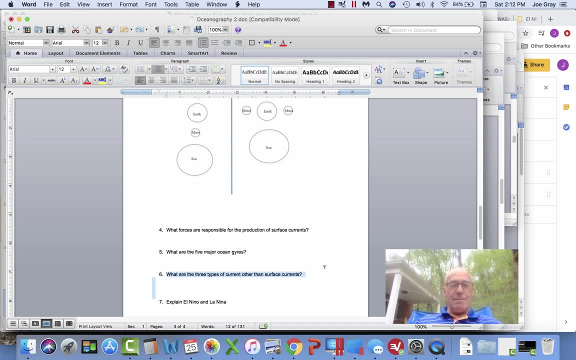 currents are what we talked about. that's primarily being impacted by wind and the Coriolis effect, But there are other types of currents as well. Let's take a look at those other three types of currents. You remember in the previous video talking about tides. So there's high. 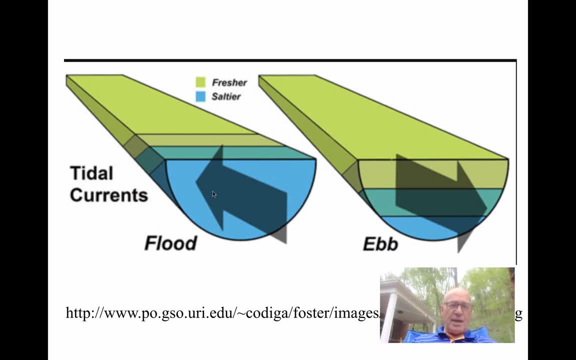 tide, low tide, High tide causes flood tides to come in towards the coast, and low tide causes ebb tides. Remember, flood is an incoming tide. Ebb is an outgoing tide. Now these will actually create tidal currents and these tidal currents- 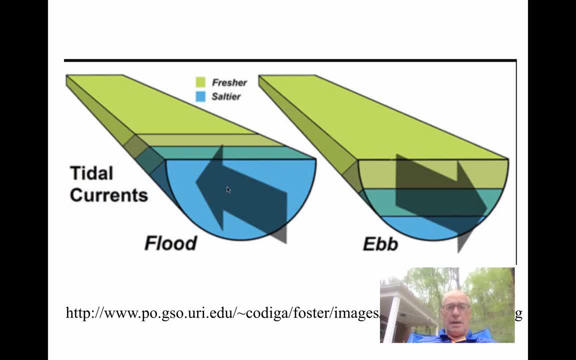 can be quite strong. They can create the rip currents that can be quite dangerous, And I remember, living in Florida, seeing signs on a causeway that was connected to a bridge going across Tampa Bay that had signs warning of dangerous currents. These were primarily tidal. 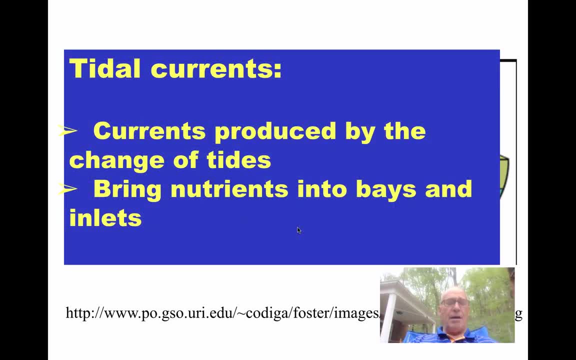 currents. So that's our first type of non-wind driven currents. tidal currents: These are currents produced by the change of tides. They're very important because they bring nutrients into bays and inlets. So you'll remember, in the previous video I showed you a little clip of a high tide, a flood tide. 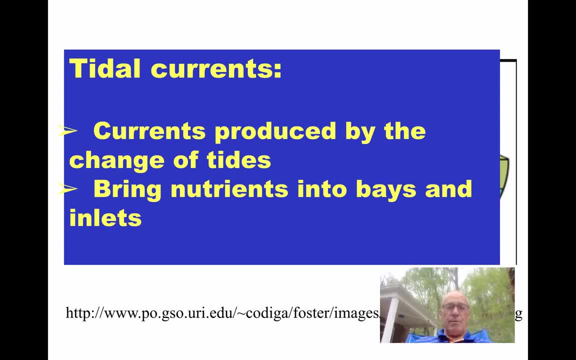 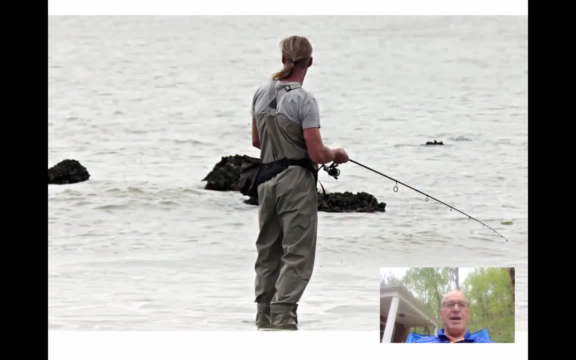 and how fish were coming into the shallow areas to feed. Well, this will also then affect fishermen. Fishermen watch the tide charts to find the best times to go out fishing. During a flood tide is the best time to go out fishing because not only are the nutrients going to be coming in to the 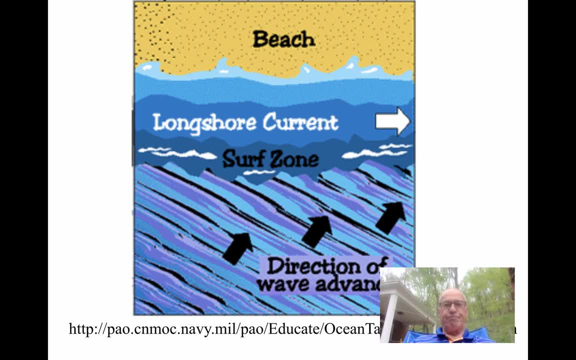 shallow waters, but so are the fish. If you've ever laid out on a beach, you may have noticed this before. Let's say, you've got your beach towel up here on this beach, right here, and then you decide to go out on a little floaty and float around there enjoying the nice warm sun. Well, that's not. 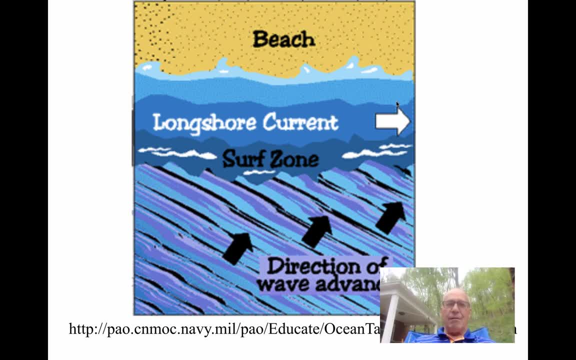 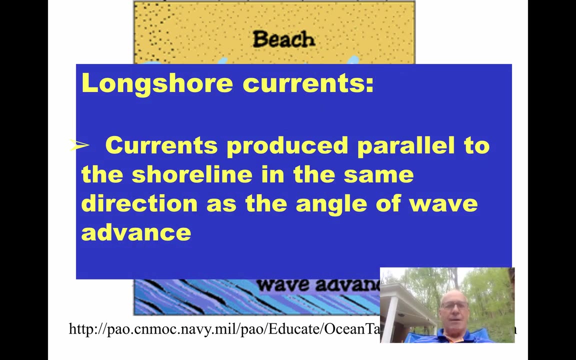 right. Well, the next thing you know is you're down here- Here's your stuff, up on the beach. You're like wondering what happened. How did I end up down here? Well, this is due to an effect called a longshore current. So a longshore current are currents produced parallel. 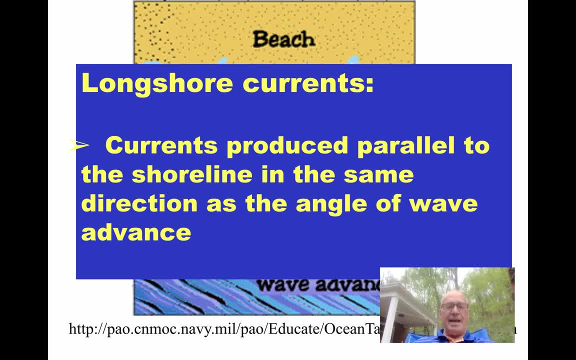 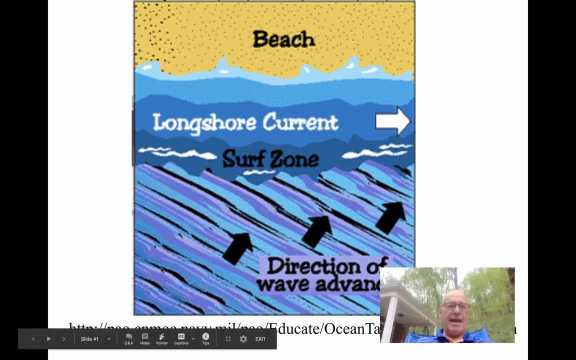 to the shoreline in the same direction as the angle of the wave advance. Now the wave advance. you can see the waves are going, coming in at an angle. They're not coming straight in And you'll notice that that's probably frequently the case. It's not too common that. 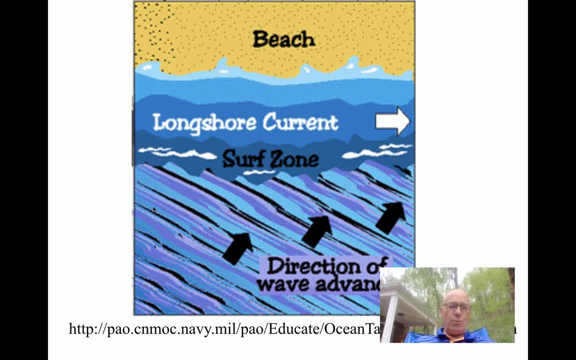 your waves are coming straight in at the beach. What they do is your wave comes in and when it bounces off, it's kind of like a billiard ball. It's going to bounce off at an angle like this And that, as a consequence, creates a current that drives the water down along. 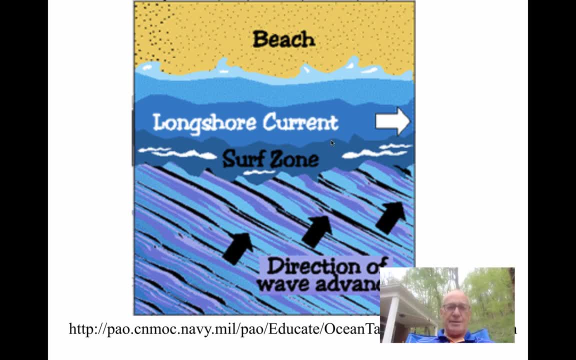 the shore. This can be very important to coastal communities. I can remember a community in Florida I live near that had built a breakwater right here. A breakwater is a pile of rocks that were going out that allow fishermen to stand on and fish. Well, the problem is that longshore, 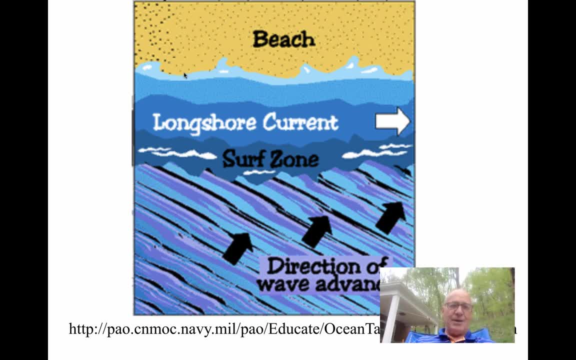 current would come along and pile up all the sand right here, Well, down on this part of the beach. that's where the sand- what we call beach renourishment- that's where the sand for this beach would have come from. So they found this community here, found that their beach was. 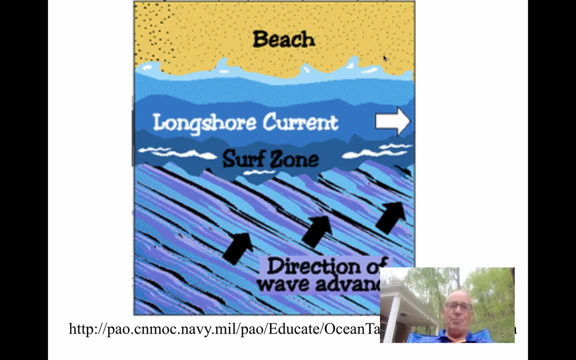 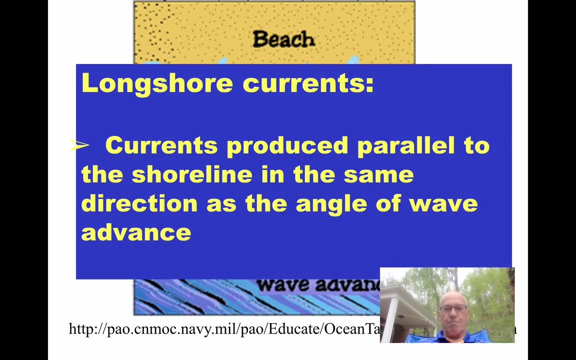 getting eroded. Well, area up here was growing new beach, so this city sued the city further up the shore to get rid of that breakwater because it was impacting the longshore current. the third type of current is called an upwelling. so here you have. 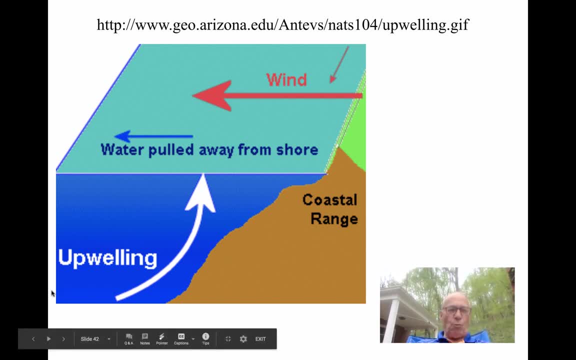 those, one of those bottom currents that I mentioned earlier. those cold water currents are coming along and now they hit a coast and that causes the water. then water has no direction other than go. the current has no direction to go other than upward. meanwhile, your wind on your surface is pulling the water away. 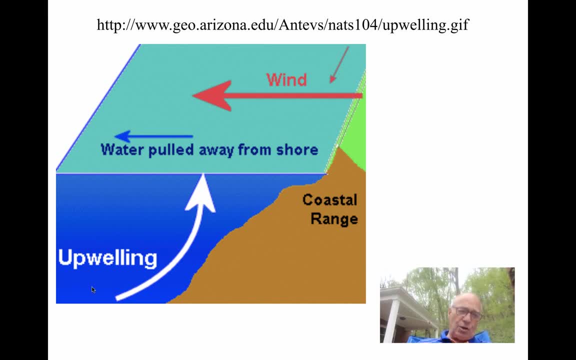 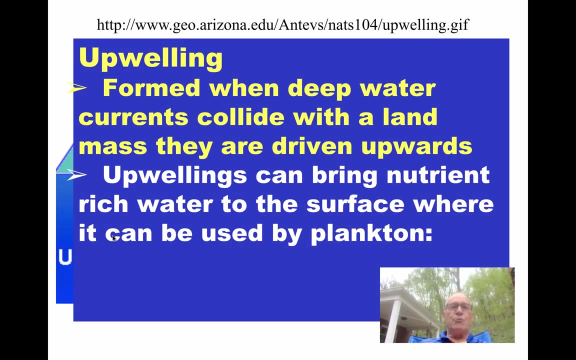 from shore, so that's creating kind of a little circle of water right here. this upwelling is very important because it's going to bring nutrients from the bottom up to the surface, where it can then be used by plants. One of the best places to see this is in the west coast, in a place called Monterey. 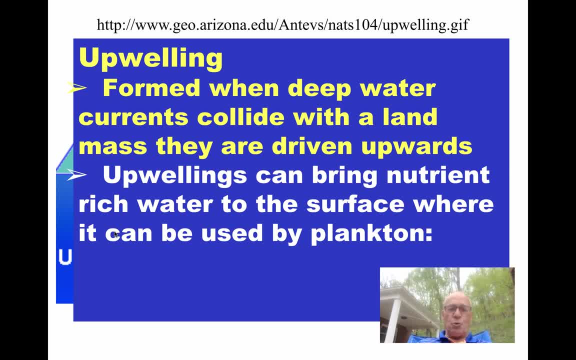 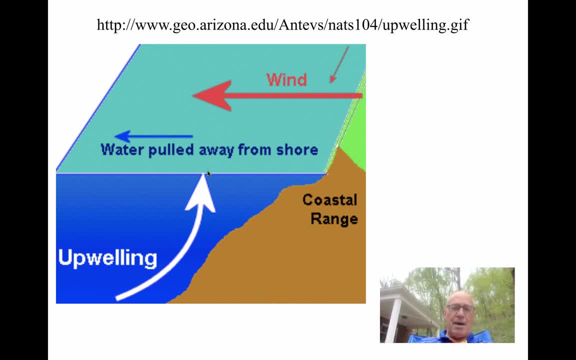 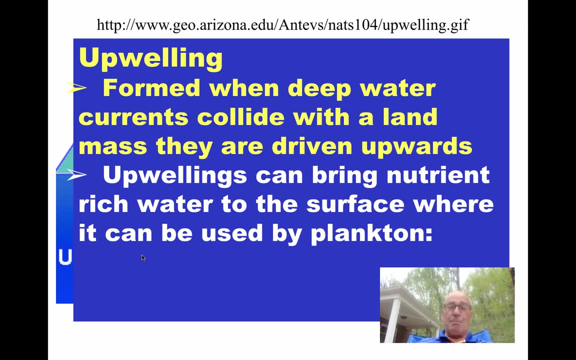 Bay. Monterey Bay has a canyon right off the shore and, as a consequence, the water comes through that Canyon. that very deep canyon comes up from the bottom, creating this very rich environment and an aquarium by the name of the Monterey Bay Aquarium. in my opinion, the greatest aquarium in the world was built there. 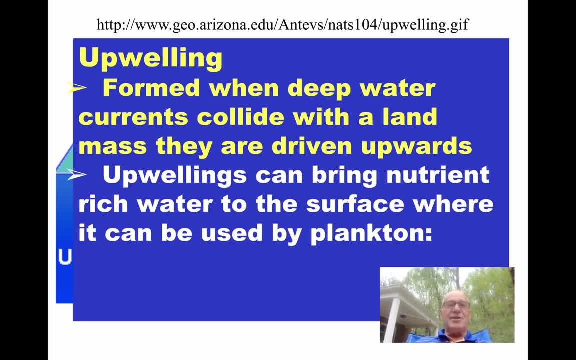 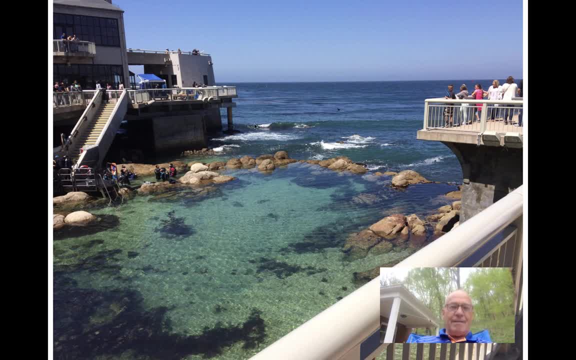 and we see all of this life being brought in to Monterey Bay right here by that upwelling current and even though this is fairly cold water, you see these scuba divers right here gearing up. they're gonna go out swim around. hopefully see some sea lions as they swim around, maybe some sea otters as 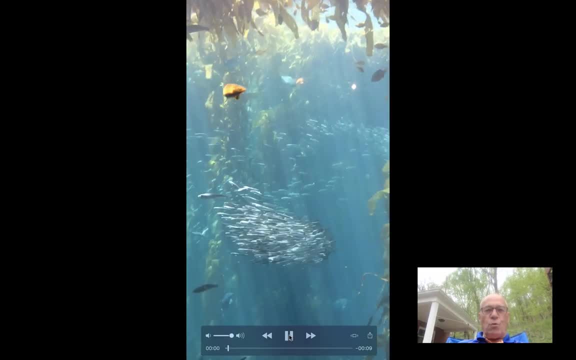 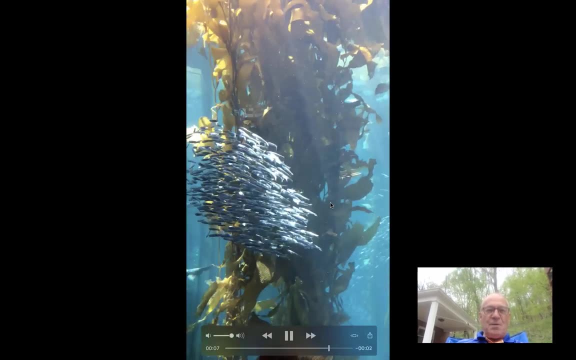 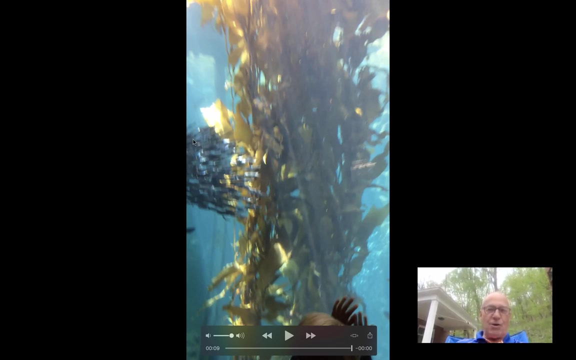 they swim around out here. one of the things that's interesting about this is that the people are looking out onto the actual Bay right here, so you can see all this kelp right here and all this sea life being brought in. so, unlike with the Newport Aquarium, where you have the 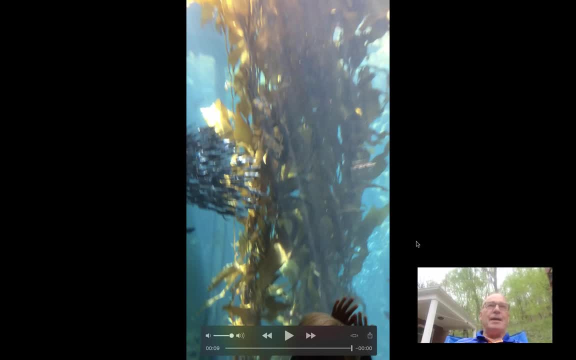 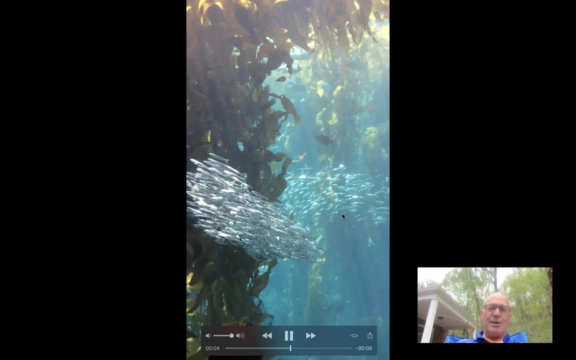 animals in caged inside of a glass enclosure and then we walk around and look at them. this time the people are kind of the caged individuals and the animals and plants are free to roam around, as we could see right here. you see a school of fish coming in swimming around this kelp. 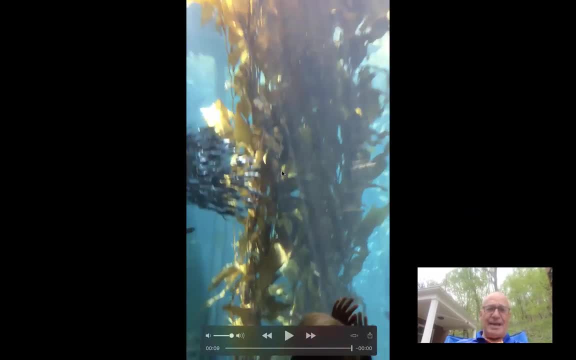 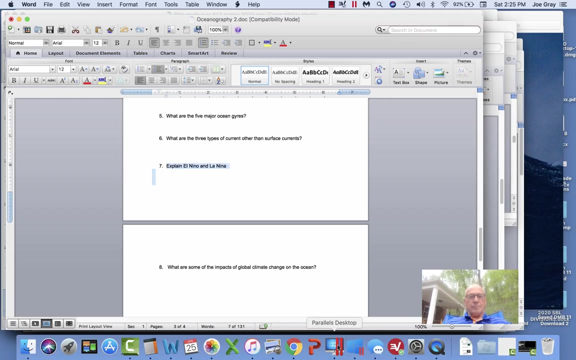 so this is actually open bay right here leading out into the ocean. this is about 30 feet down, about 30 feet under water, looking up at all of the life that's brought into this Monterey Bay Aquarium. our next question, to address question number seven: what100 does the Monterey Bay Aquarium offer to someone who is starting? 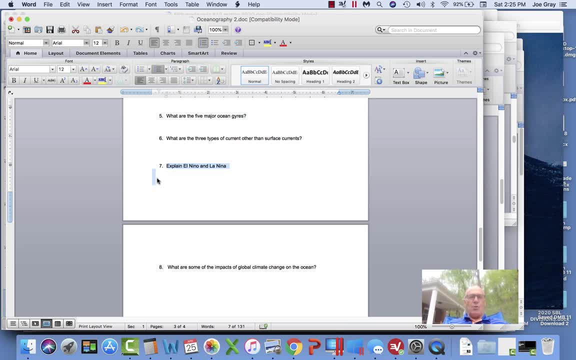 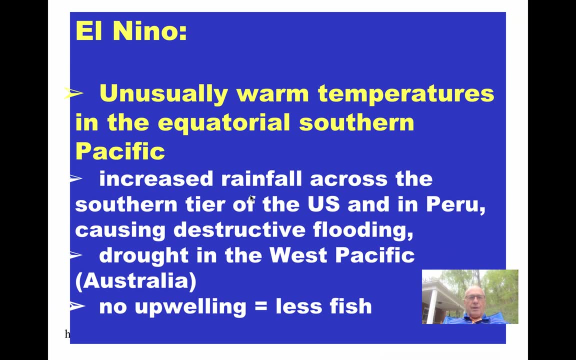 effects known as El Nino and La Nina. Again, these also have to do with ocean currents. Let's take a look at El Nino. El Nino is when we have unusually warm temperatures in the equatorial southern Pacific. So this is along the equator in the Pacific, And this causes 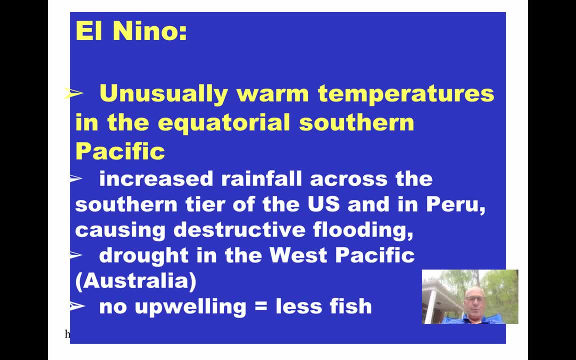 increased rainfall across the southern tier of the US and in Peru, And that can cause some pretty destructive flooding. This also causes drought in the West Pacific, such as Australia Now. remember those horrible fires that Australia had this past season, That's. 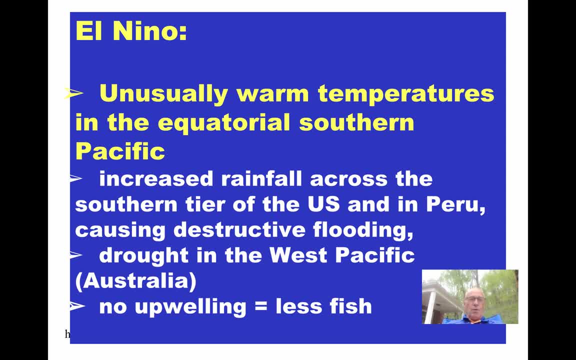 a consequence of the effect of El Nino. With El Nino there's no upwelling Because of the warmer water. the colder water is not coming up from the bottom And remember that brings nutrients up, so there's less fishing And this is taking place primarily in South 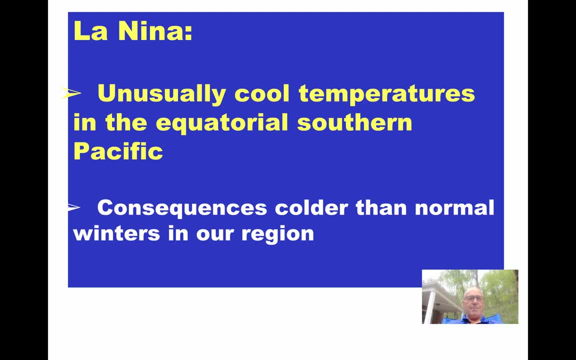 America. La Nina is when we have the opposite, usually cool temperatures in the equatorial southern Pacific, And the consequences are that we have colder than normal winters in our region. Well, you saw this past winter. We definitely did not have a colder than normal winter in this. 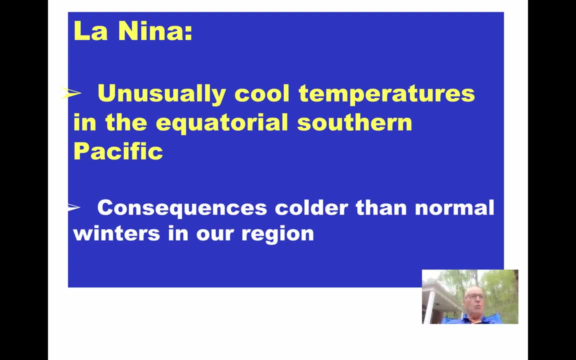 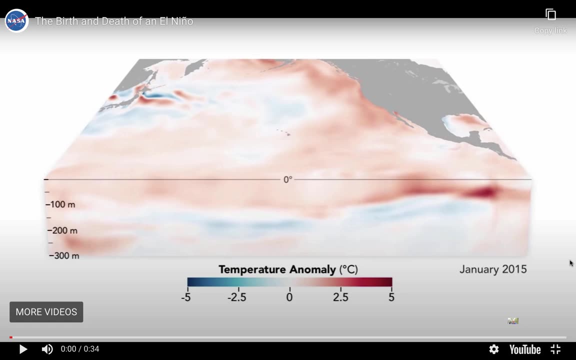 region. Let's take a look at a National Oceanic and Atmospheric Administration video that, hopefully, will help you understand the concept of El Nino and La Nina a little better. This video clip you will see starts in January of 2015.. And you can see how the temperature. 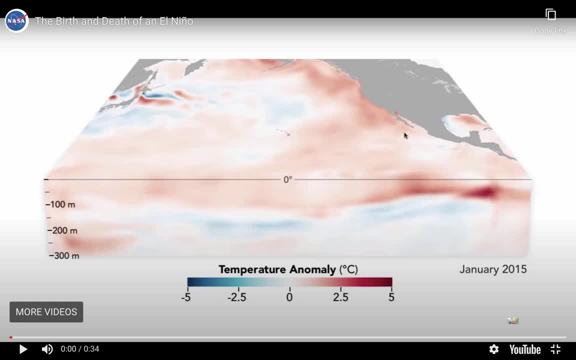 changes across the Pacific. Right here is the west coast of the United States And down here we're getting close to South America. It's going to be over here on the far right, just out of view of this. Temperature anomaly means the difference in what the normal temperature. 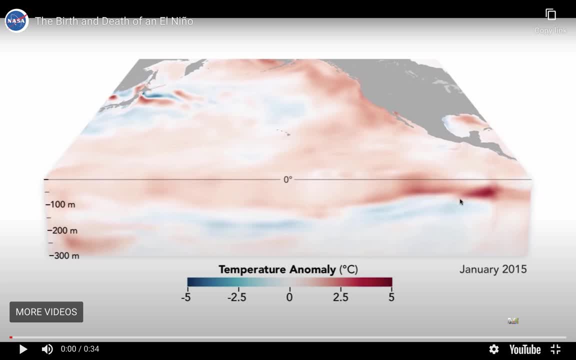 would be. So zero would be what the normal temperature of the ocean is in this particular area right here, And then the colors show how far above normal or how far below normal those temperatures are. So let's take a look at what's happening in the video here. So here we can see. 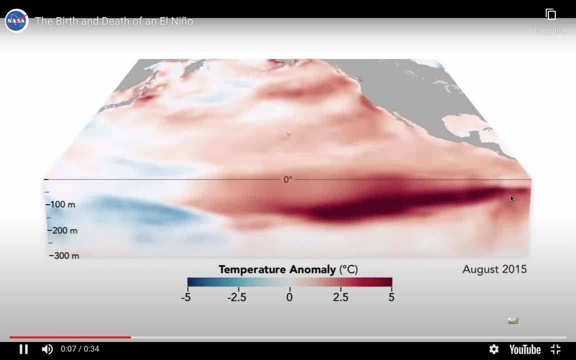 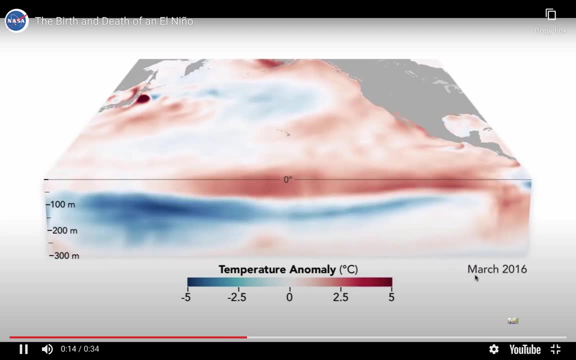 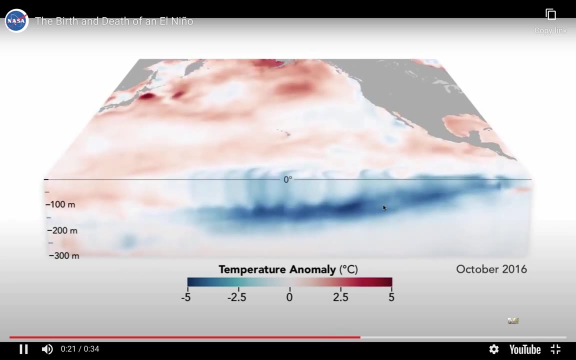 an El Nino. Look at how much warmer this temperature is getting here as you get close to South America And we get into December of 2015.. And now El Nino is going away and we're switching to a La Nina. Notice, the water's like going the opposite direction here. We've changed our 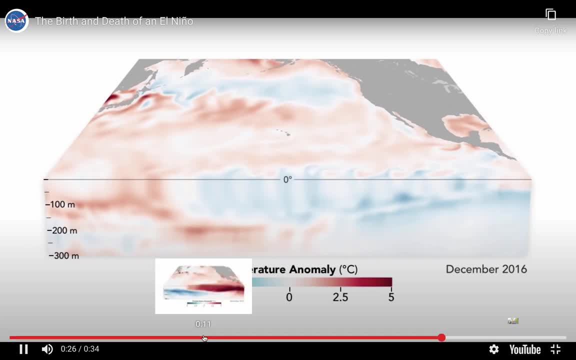 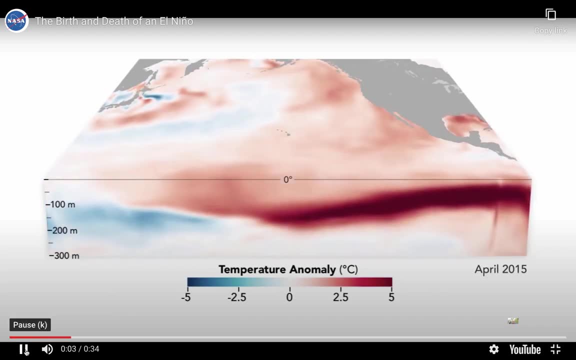 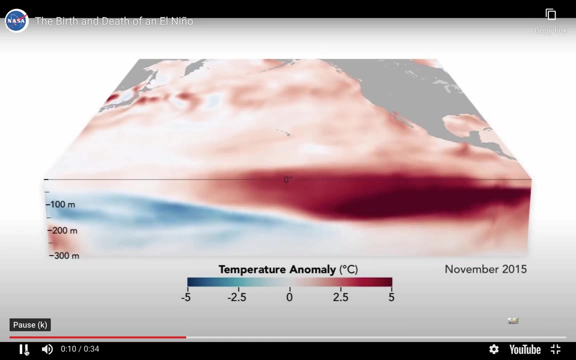 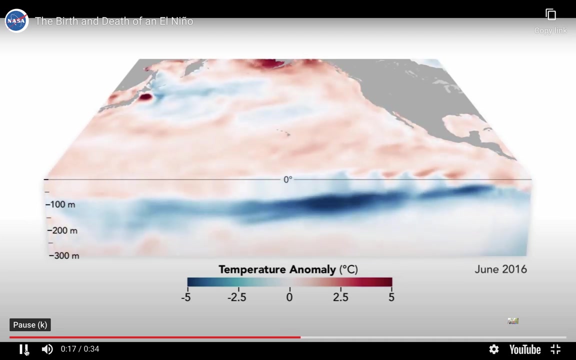 direction and our temperatures drop below normal. So we've gone through both an El Nino and a La Nina. Let's see that again: El Nino, La Nina. Our last question to address in your notes here is question number eight. What are 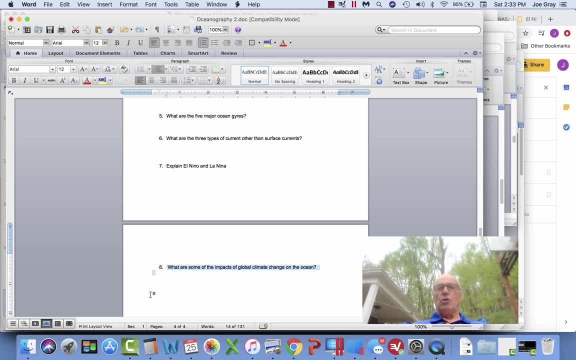 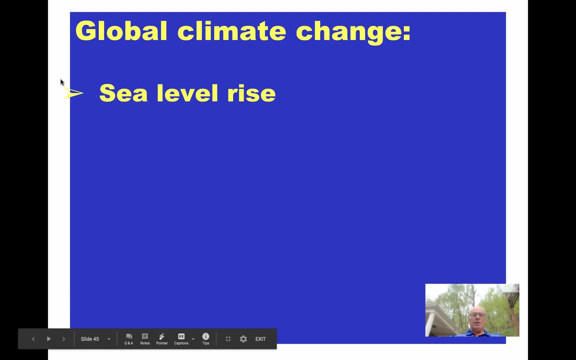 some of the impacts of global climate change on the ocean. Let's take a look at those impacts Now. the first: you've probably heard of the word climate change. It's a term that's used a lot in the United States. It's a term that's used in the United States. It's the term that's used in the. United States, But right now, we're talking about a global climate change. Now, climate change is a term that's used in the United States. We're talking about global warming. It's a term that's used in the United States. It's a term that's used in the United States. But what we've probably 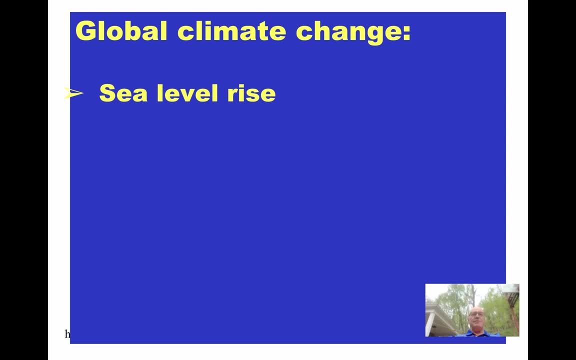 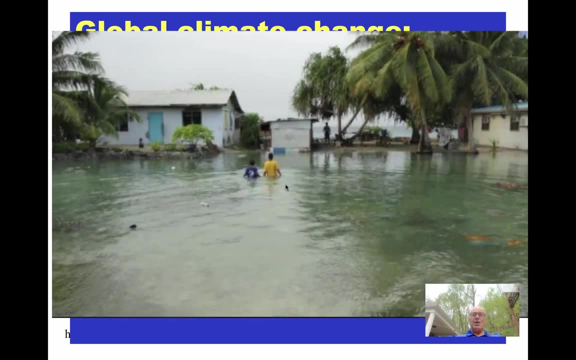 already heard about. in many cases is sea level rise. We're seeing the evidence of sea level rise, world rise, in Pacific Islands especially. This is high tide now. Now, obviously this is not normal. These people did not build their homes in an area where there would normally be water covering up. 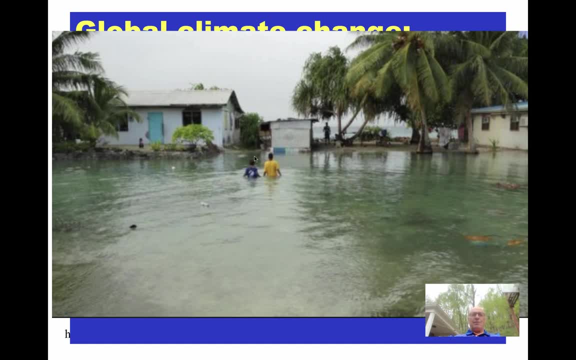 the walkway to get to their homes. This has happened in the time since these people made their. These people are becoming homeless. They're being forced out of their homes and off of these islands because they're being flooded. These are the Marshall Islands in the western Pacific, which are protected by the United States. 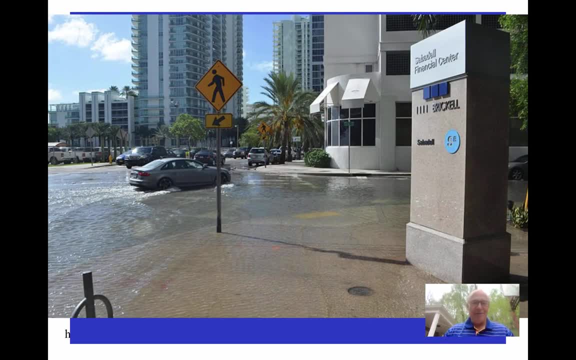 This is the United States, This is Miami, and this is a high tide that's actually flooded the streets. now, Is it normal to have saltwater out on your streets that you're driving through or walking through? No, it isn't, But this is happening with increasing frequency in low-lying cities like Miami, cities that are close to the coast. 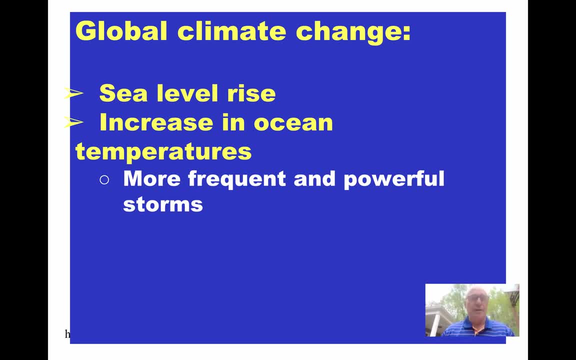 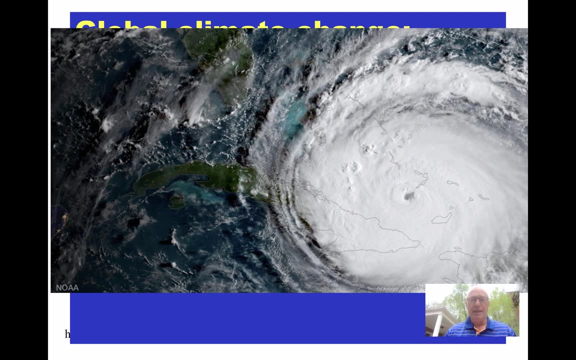 The second effect on global climate change is obviously an increase in the temperature. the Earth is increasing, so are the ocean temperatures, And what that does is that causes more flooding, More frequent and more powerful storms, such as hurricanes. So here we see a satellite view of a hurricane heading for the United States right here, right off the coast of Cuba. 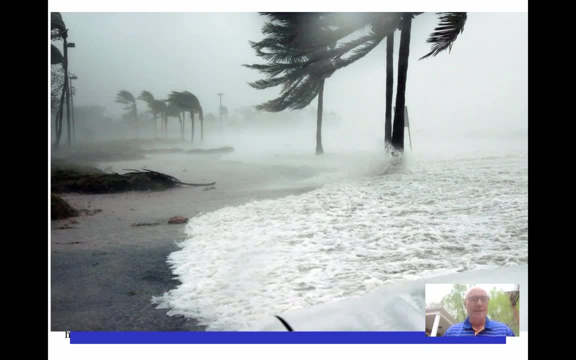 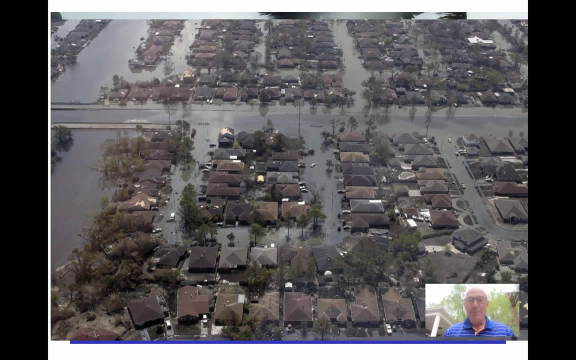 These can be quite destructive. as you've probably seen in the news, Hurricane Maria, which hit both Puerto Rico, which is a United States territory- The people who live in Puerto Rico are American citizens- And then it also did quite a bit of damage in Florida. 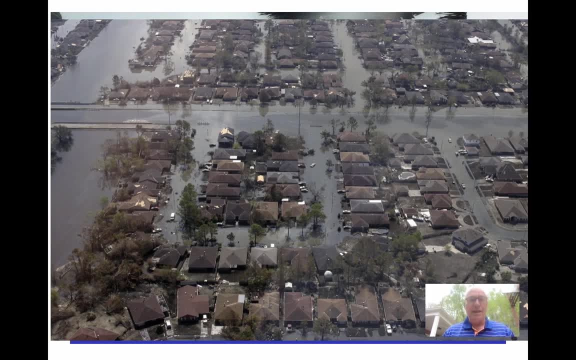 This is the flooding that we saw in a place such as New Orleans. This costs billions of dollars. It costs lives, which are really even more important, But it's something we all, as adults, will have to pay for through increased taxes in order to take care of the damage. 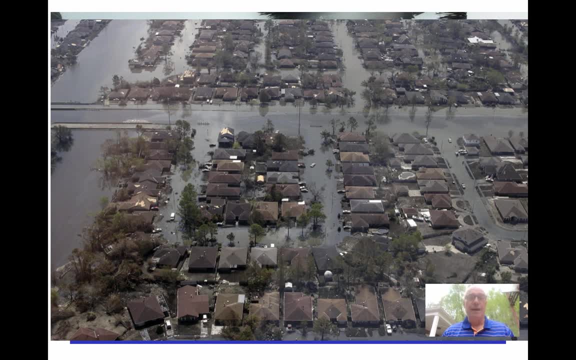 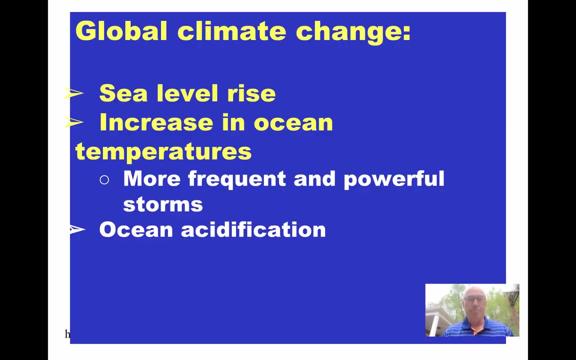 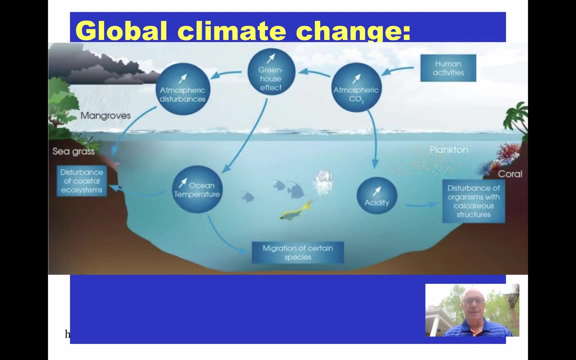 And those people who live in areas like this are going to have to pay. They're going to have to pay higher insurance costs in order to protect themselves from this kind of damage. The final problem is ocean acidification. Now, what ocean acidification does is the higher the acidity of the ocean, the less likely organisms who make like coral, who make skeletons from limestone, calcareous material, are able to do so. 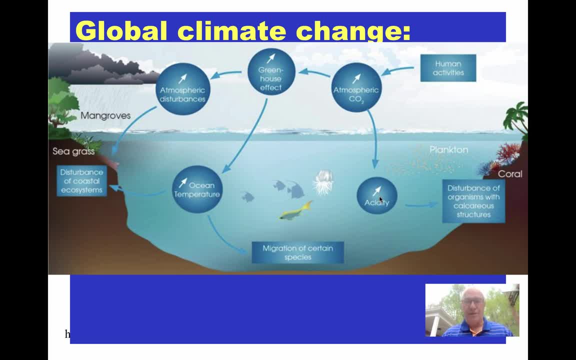 Because the ocean acidity Dissolves the calcium that's in the ocean, making it unusable by these organisms who are not able to use it, And it's the carbon dioxide which is your primary cause of global climate change in the atmosphere. that's increasing the acidity of the ocean. 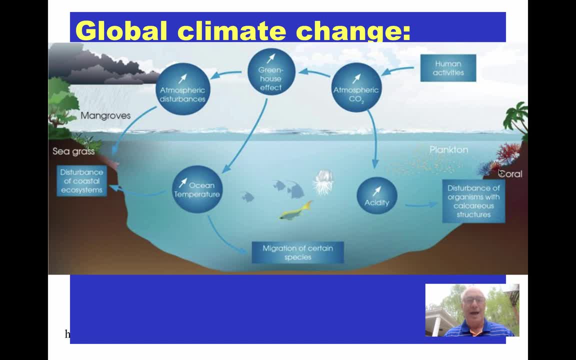 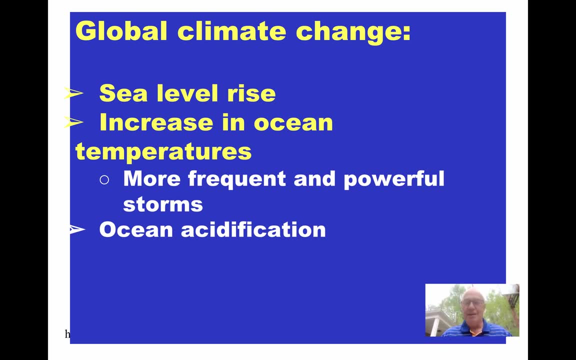 So, consequently, we're seeing a worldwide coral die off. These are all problems that you, as young adults, are going to have to address as the climate changes, And hopefully we're going to find some ways to deal with that. Alright, so this is the second and final video applying to oceanography. 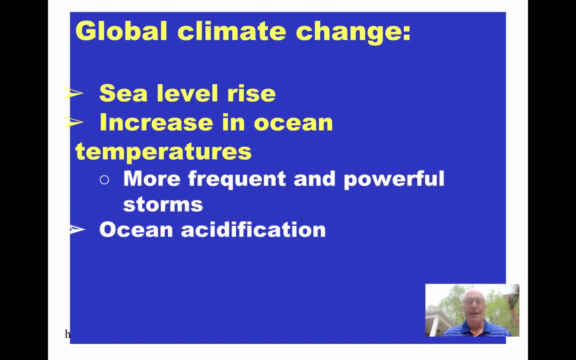 Remember that your completed notes are due next Wednesday, That's April 29th. There will be a follow-up quiz, but that will be coming the week of May 4th. Please make sure to contact me if you have any questions. Thank you. Thank you.